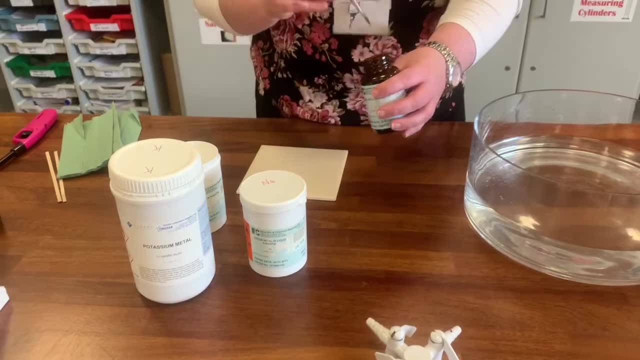 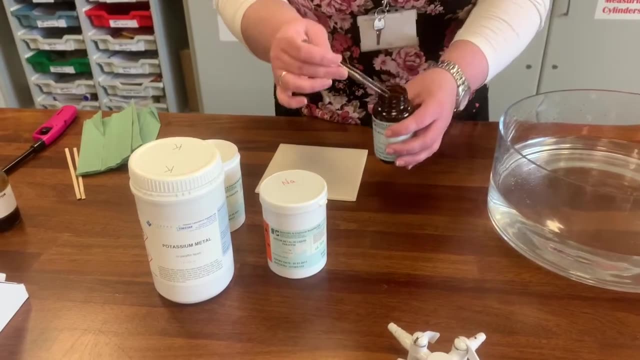 reacting with any moisture or any oxygen in the air. So whenever we want to take a sample of the metal, we need to fish it out of the oil, which is not very easy. Okay, there's a wee tiny bit and we're going to use a paper towel and we're going to make sure all the oil is wiped off. 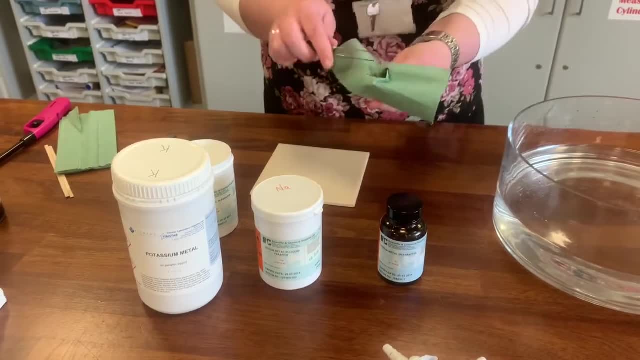 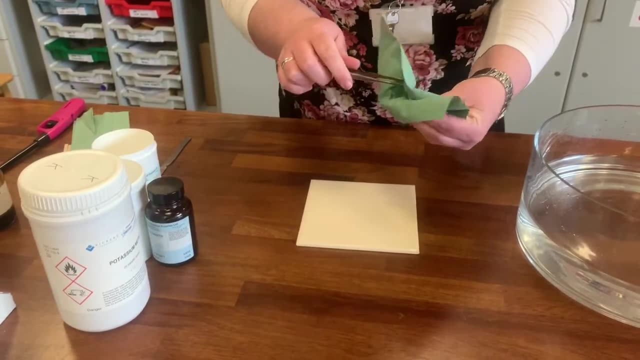 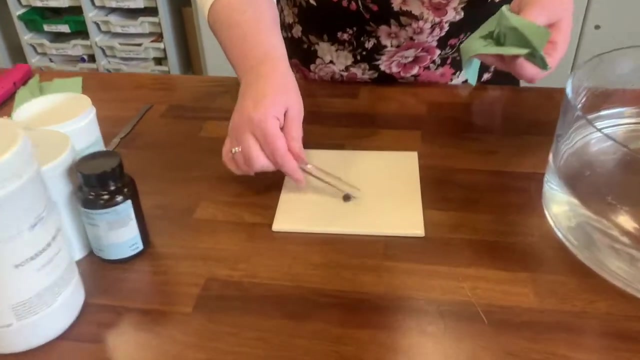 and then put the lid back on. So we've got a little tiny bit of metal. It's not what you would expect for a normal metal. So if you ask me to describe a normal metal, we might not describe what lithium looks like or sodium or potassium. So you'll see it's actually quite dull. It's very easy to cut, but watch when. 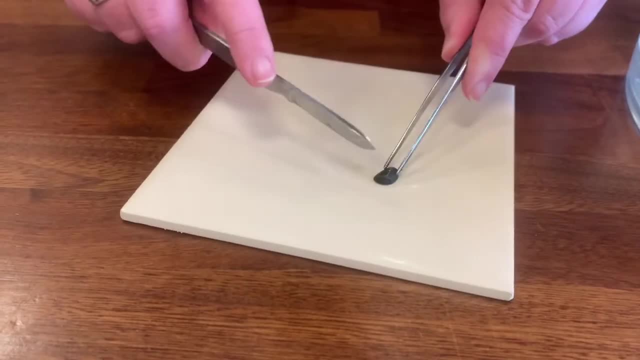 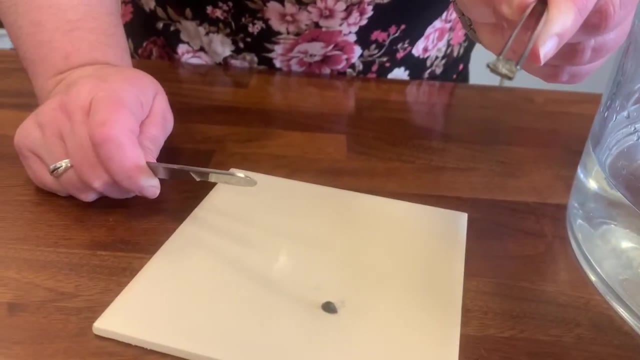 I cut it to see. when I cut it it's actually quite shiny inside, but then it quickly goes dull. So easy to cut. and then it's shiny and then it goes dull once it reacts with the oxygen in the air. Okay, most metals don't do that. Most metals you can't cut with a knife. 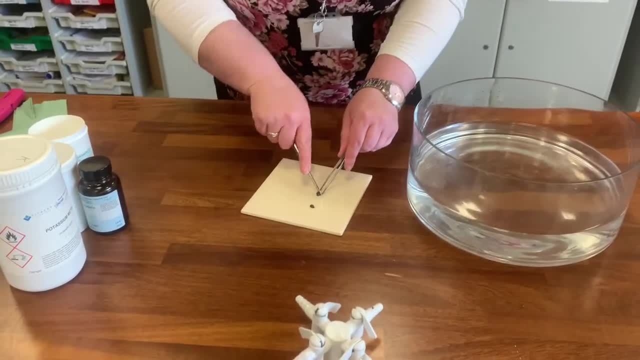 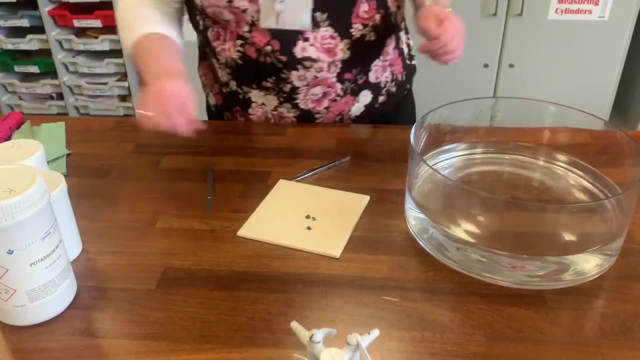 whereas group one metals you can. So I'm just going to cut this up into another piece and then show you these pieces reacting with the water. So put the lid on that one. Now. lithium is at the top of group one. It's in group one, period two. Remember, if you've done, 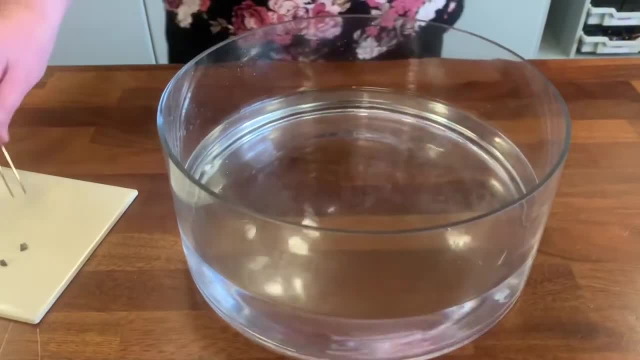 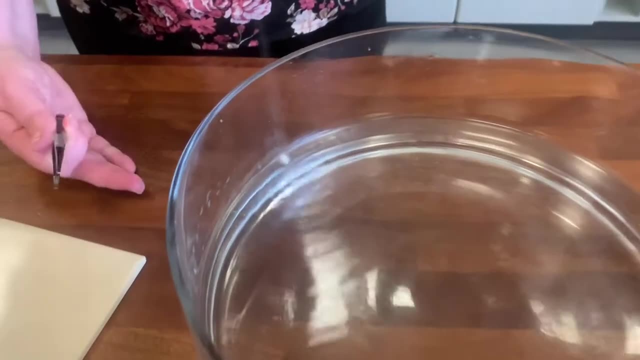 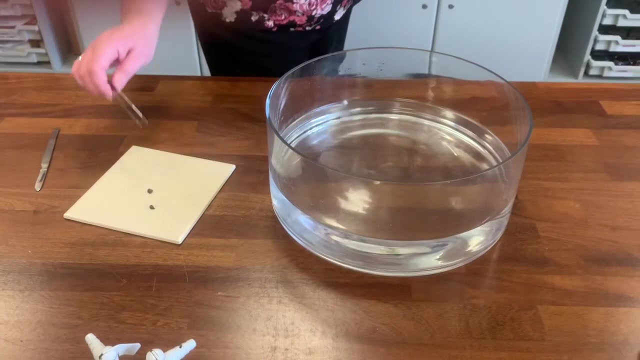 that. So once it goes into the water, it floats on the water and it immediately starts to fizz. So our observations for this reaction is that the lithium floats, It fizzes. You can really hear the fizzing in the bubbles. It moves around on the surface of the water and it just disappears. The metal's getting smaller. 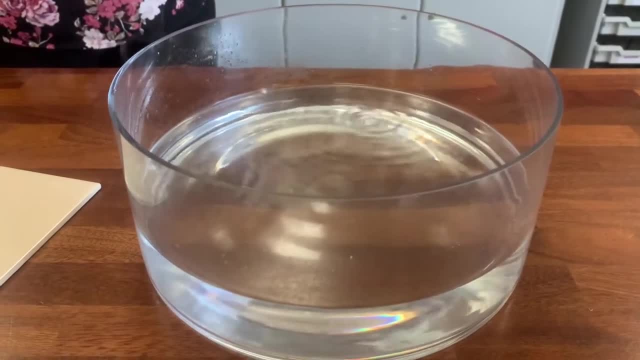 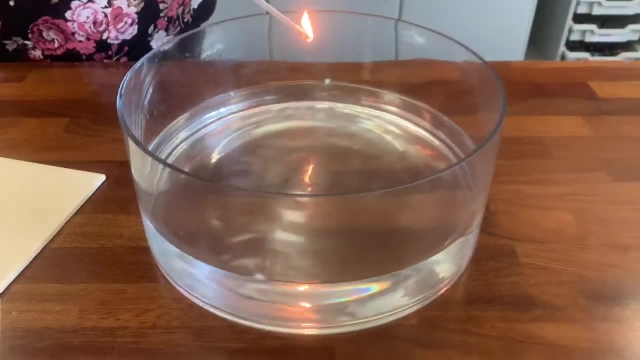 The gas that it's producing is hydrogen. So if you think back to your work, where we're testing our gases, The test for hydrogen gas is it burns a squeaky pop. So I'm just going to try and prove that this is hydrogen. So listen to the pop. 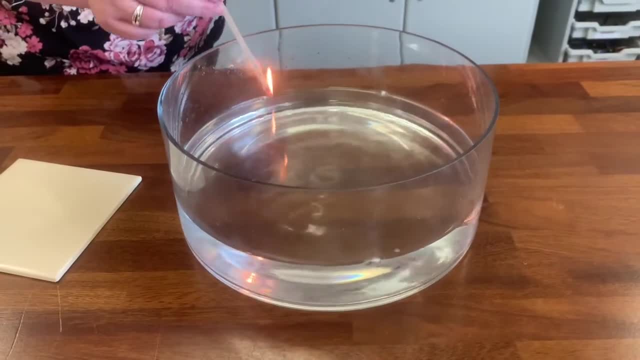 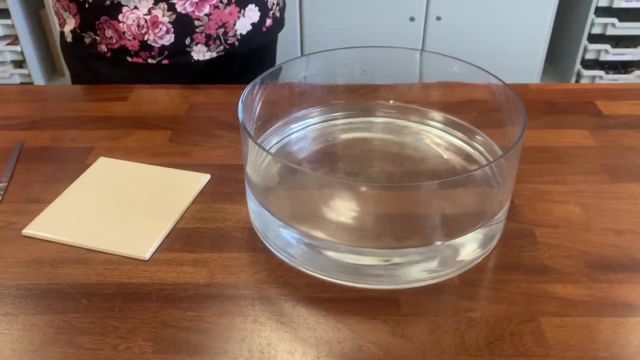 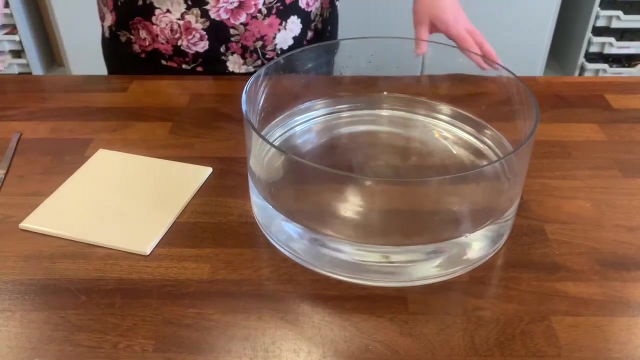 Okay, so that proves to us it's hydrogen. Now that isn't an observation for this reaction. The observation is just that it's fizzing. So remember, an observation is what you see, what you hear and what you feel. So I'll go over those observations again because you maybe need to write. 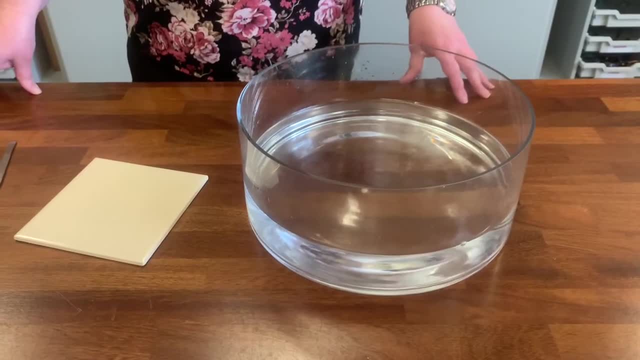 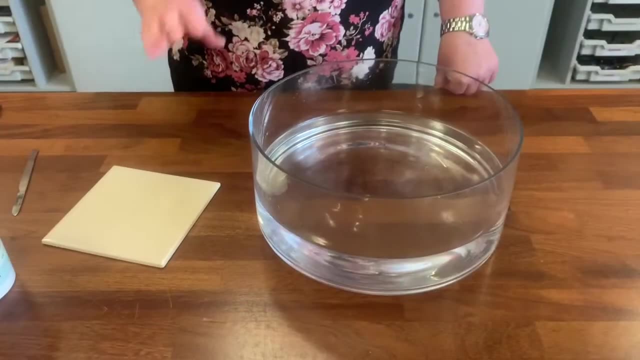 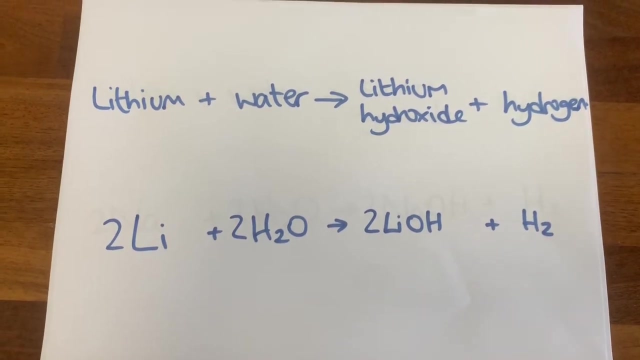 those in your booklet. So the lithium floats on the water, It fizzes, It moves around the surface and then the lithium gets smaller. Okay, So those were the observations. when lithium wrecked water. The equation is so: lithium plus water produces lithium hydroxide plus hydrogen, and the symbol equation is written underneath. 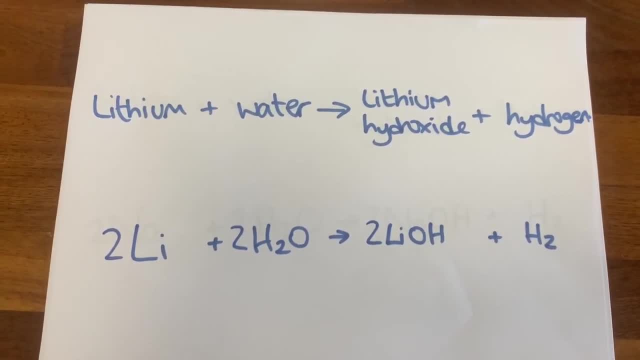 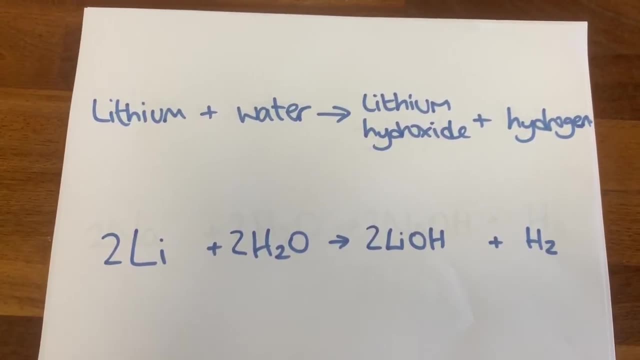 Now, at the end, once I've finished reacting all these metals, I'll show you what it means to have a hydroxide produced. So these are called our alkali metals, because when they wreck the water they produce an alkali. So lithium hydroxide is an alkali, but we'll also do it whenever we have. 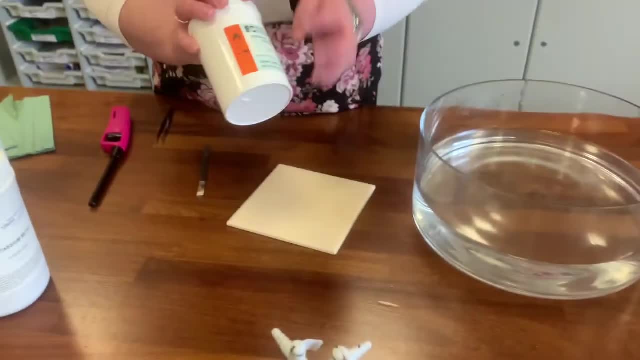 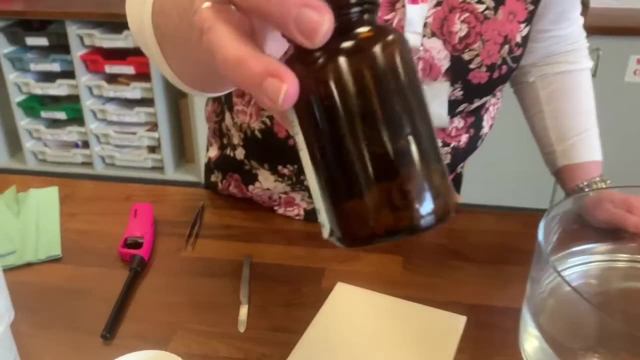 sodium and potassium. So now I'm going to show you what happens when we react to sodium. Again, it's the same type of container and inside the plastic container is our bottle. and we've got oil in our bottle again and the sodium this time is at the bottom of the oil. I wonder if you can see it in. 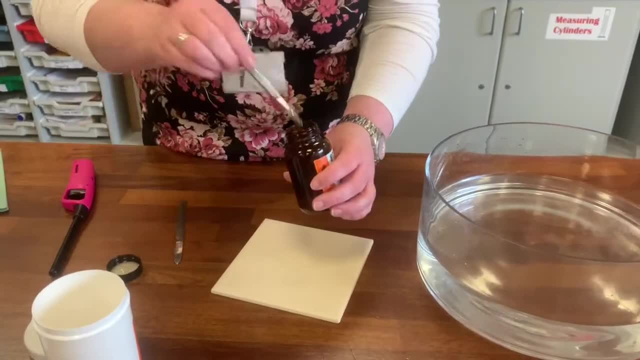 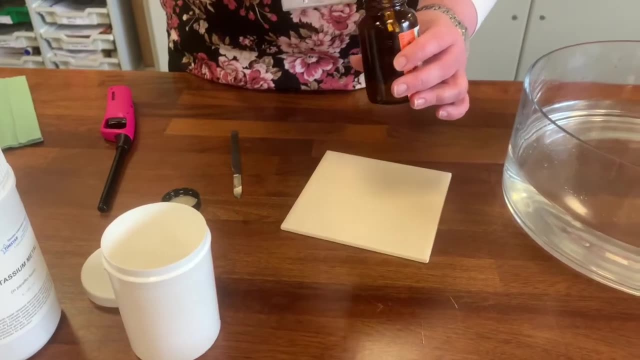 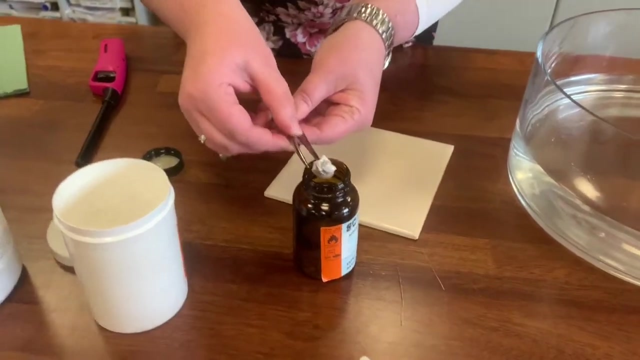 the video or not? So again, we're going to use the tweezers to fish out a bit of sodium. Now actually watch what the difference is between the lithium and sodium, because what I can do with the sodium is I can stick the tweezers in it. I don't even need to hold it with the tweezers. See, there I'm. 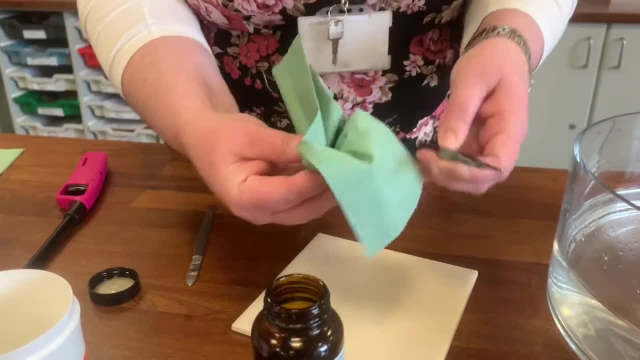 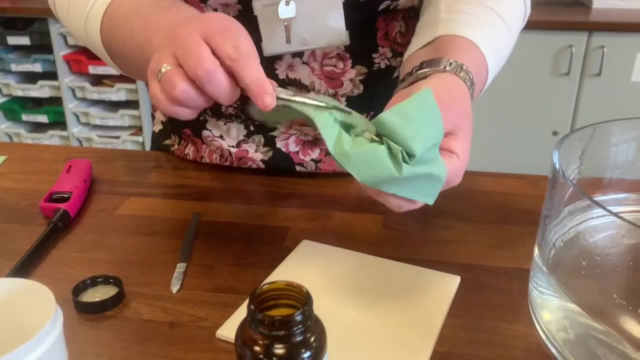 sticking the tweezers in it. So most metals aren't that soft. I'll probably lift it out more than one bit here. So remember I'm drying off all the oil. It's one of our safety precautions and our risk assessment that we have to dry off all the oil. So maybe at the top of the page you have. 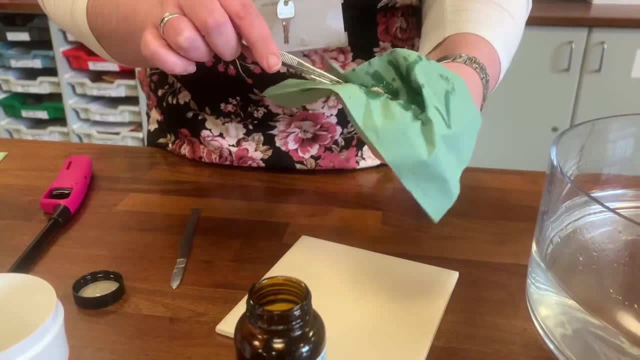 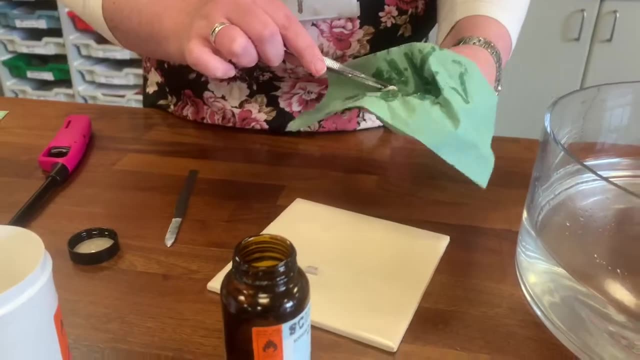 to fill in your risk assessment for this. So this is one of the bits about a risk assessment. We don't want to have oil on the metal still when we put it into the water, because we know that oil and water don't mix. So there's a little bit with the oil wiped off it. I'm gonna get another tiny bit. 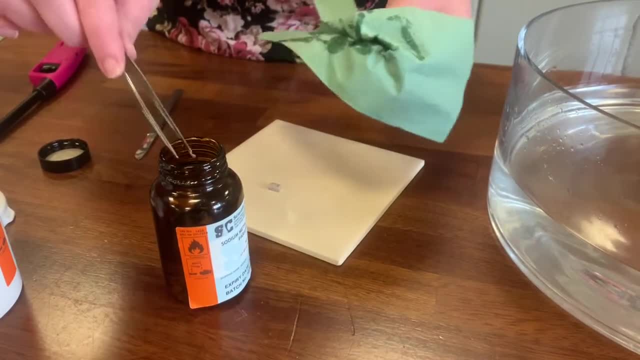 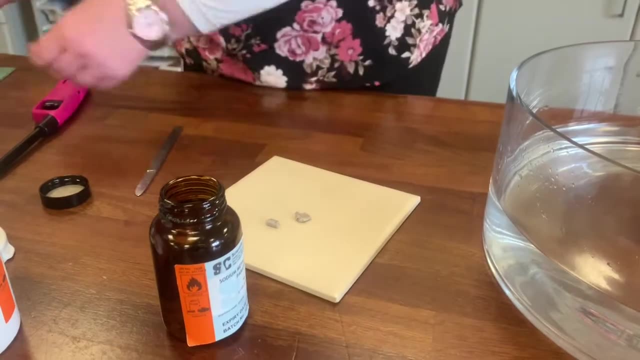 So sodium is really soft. I'll put that bit back in the bottle, Try and dry a bit with a paper towel. Make sure all that oil is off. Okay, now again it can be cut with a knife. So it's quite. it's sort of a. it's a dull colour at. 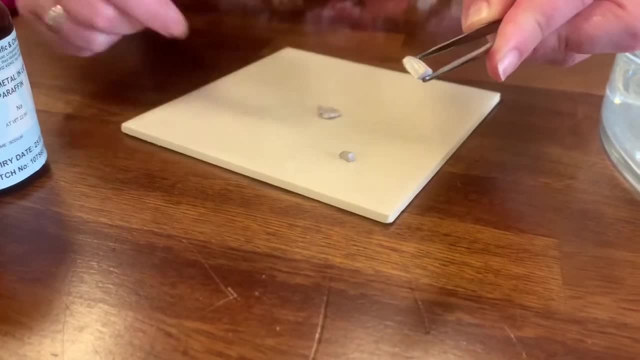 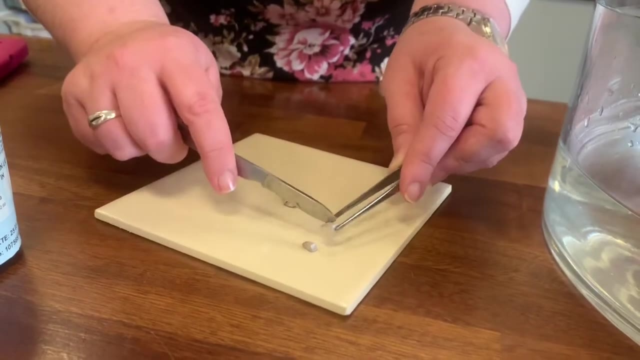 the minute and watch what happens. It goes shiny, It goes dull a lot quicker than the lithium did. So it reacts with the oxygen, but it reacts faster with the oxygen than the lithium did. Okay and same with this one, Really easy to cut. So let's have a look at what 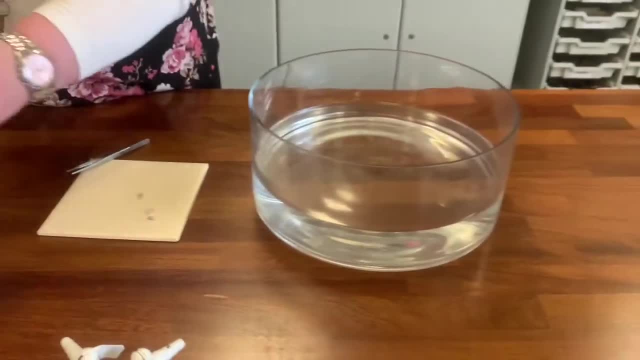 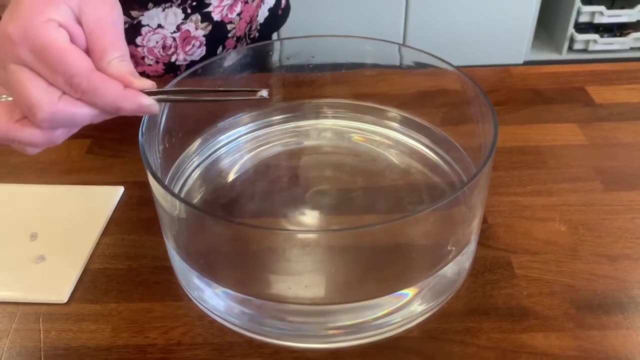 happens when we put sodium into water. So, again, we're writing down our observations in your book. So I want you in particular, to pay attention to the shape of it is at the start, once it hits the water. So have a look at the shape it's turned into. 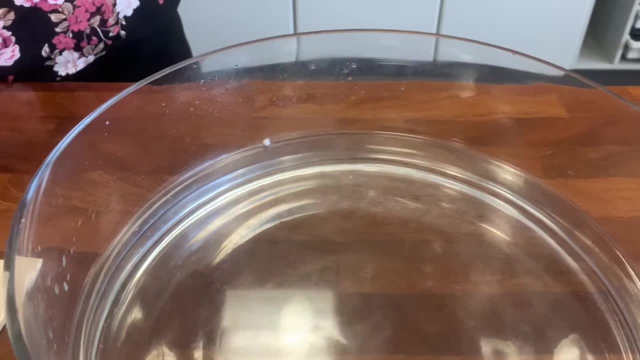 So one of the observations is that sodium melts into a ball, it fizzes and again it floats on the surface. Now the sodium has a particular movement around the surface of the water and we'll see if we can get it with this next time. 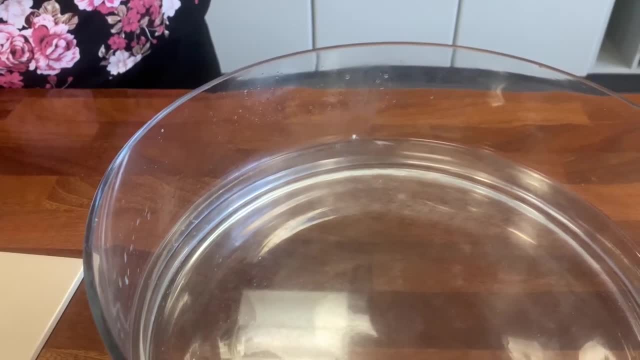 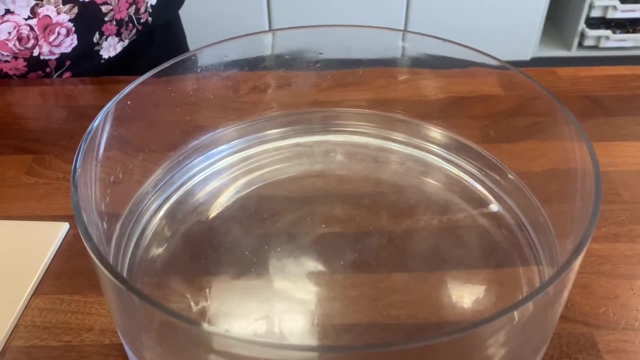 Now the sodium has a particular movement around the surface of the water and we'll see if we can get it with this next time. So again, look at the shape. I'm going to try and drop it into the middle now, So it melts into a ball and the movement is described as it zigzags across the surface. 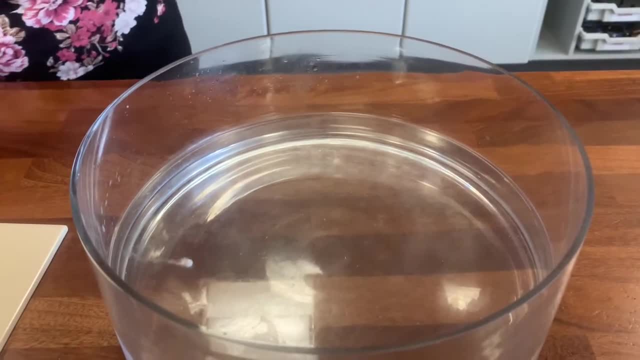 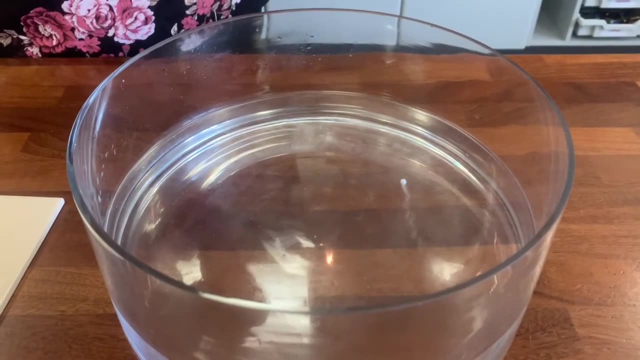 So it goes in straight lines, hits the side of the bowl and then it zigzags across Again, the gas that's being produced. they can just confirm it's hydrogen by seeing if it burns the squeaky pop. Listen to the pop. 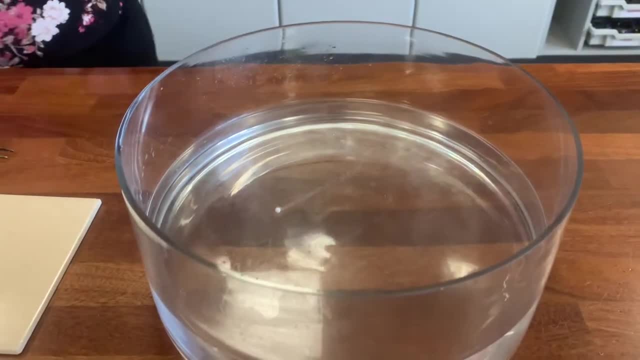 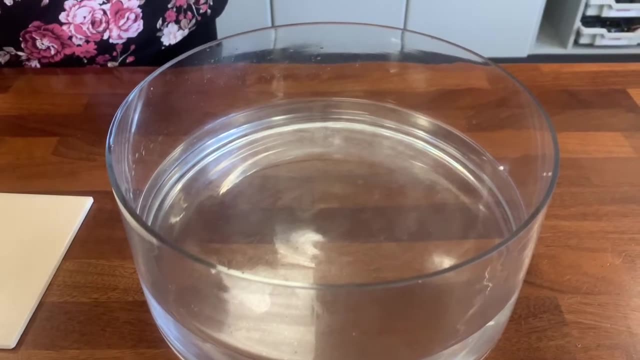 I don't know if you heard that very well. We'll try it with the next bit whenever it's a bit bigger and see. So our observations: it fizzes. This will even get smaller. It zigzags across the surface of the water as it floats. Those are our observations. 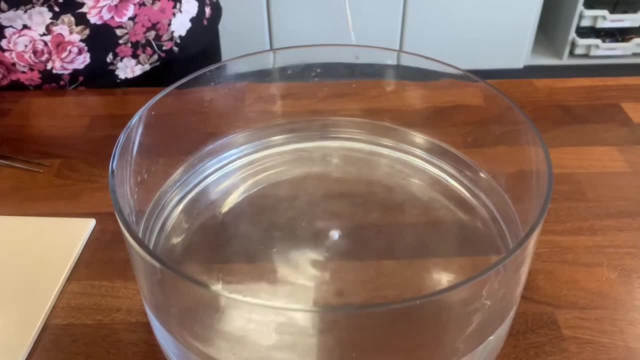 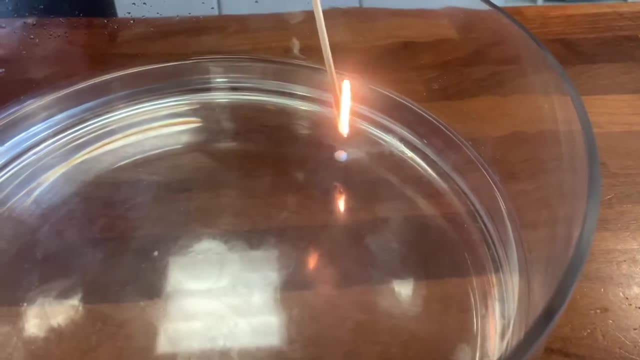 And then the last bit. So see the way it's just melting into a circle. It didn't start off as a circle. It's pretty close. Let's see if we test it, see if it's going to burn the hydrogen. Maybe it'll burn into the squeaky pop. 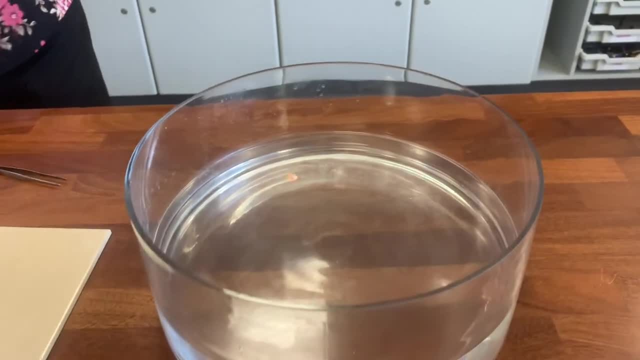 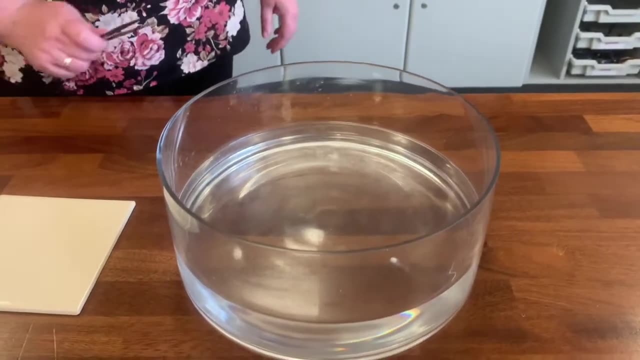 Now it's standing on fire because that's the hydrogen that's burning. So that's not part of the observation of the reaction. So the observation of our reaction again is the fizzing. This time you can maybe see the water's getting a wee bit cloudy underneath. 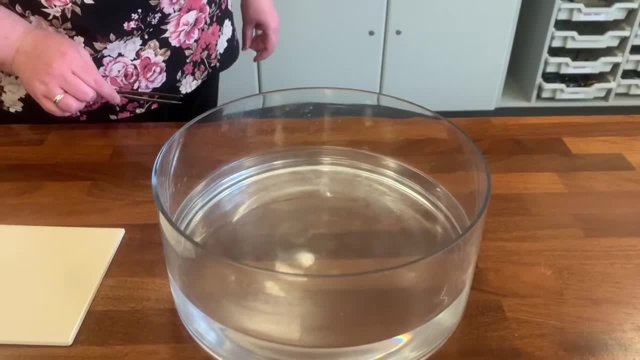 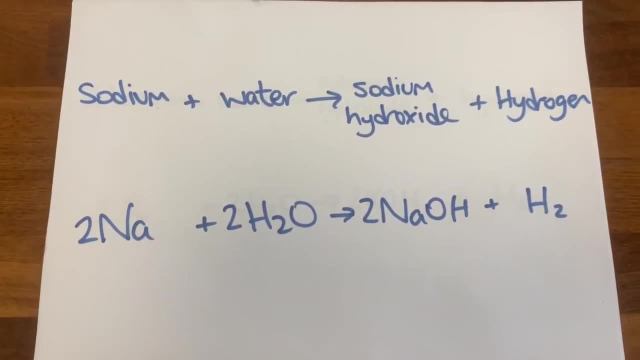 It wasn't doing that with the lithium, but it is with the sodium. Okay, so our reaction then? our equation for sodium is the same as lithium. We've got sodium plus water. goes to sodium hydroxide plus hydrogen, And there's a symbol equation underneath as well. 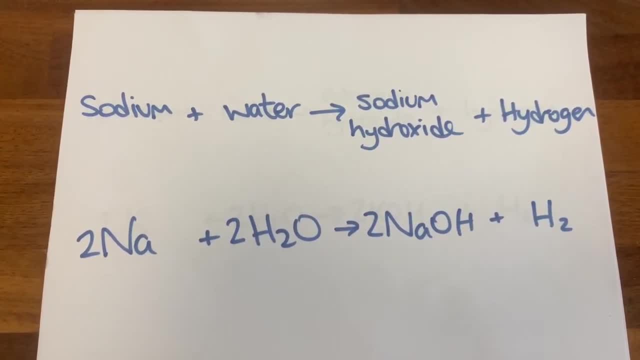 So, remember, sodium hydroxide is an alkali as well. And then our last one I'm going to show you is potassium hydroxide. So again, we've got our hazard symbols on it to tell us that we have to be careful. 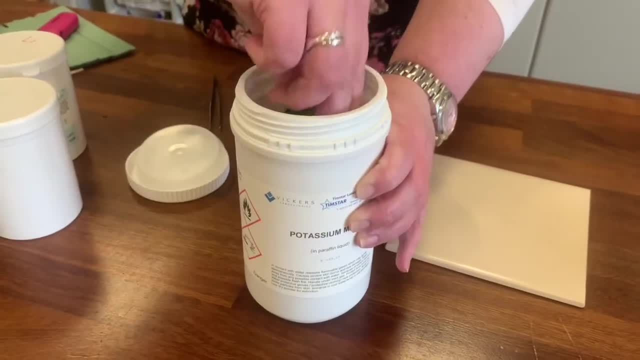 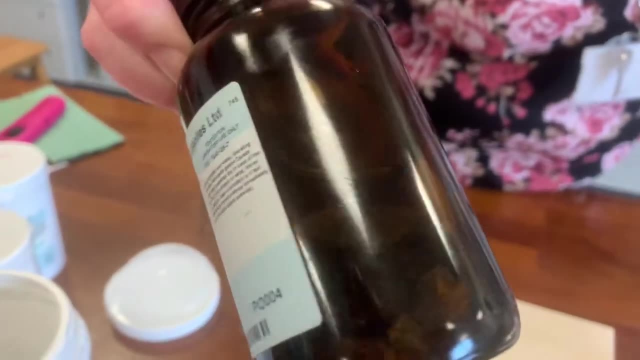 Have a look at the difference between the storage. This one is more reactive. As we go down grip one it gets more reactive. So again we've got oil in the bottle. Not sure if you can see. there's some chunks of the potassium at the bottom. 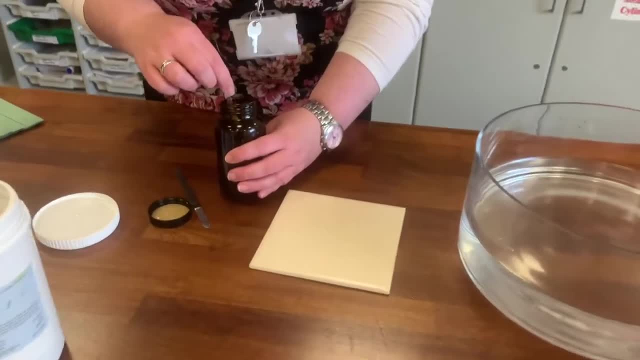 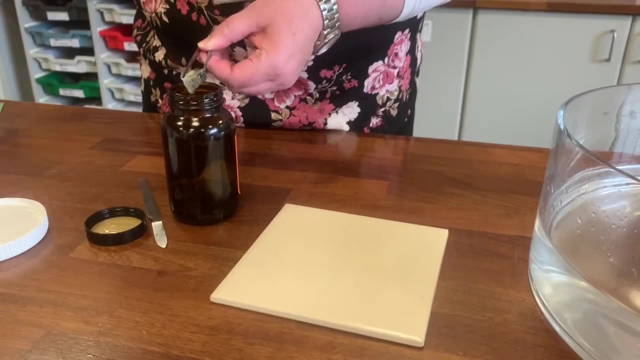 So what do you think? Do you think I'm going to be able to stab this with the tongs the way I did the last one, And if I bring it out, get my paper towel ready? So you see, I did just stab it with one bit of the tong. 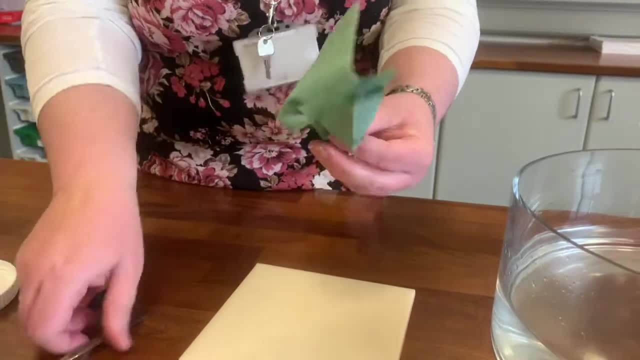 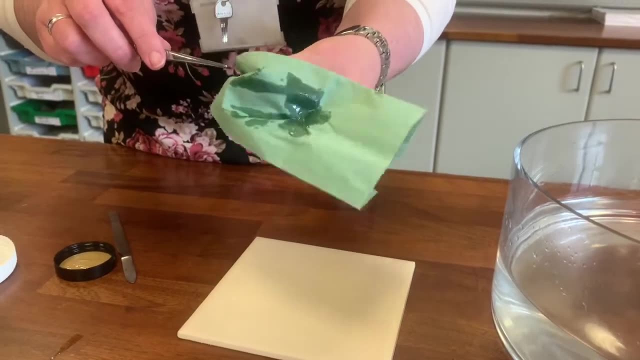 So again, it's very soft. It's not. these group one metals are not like normal metals. They don't have the normal properties. So our properties of our normal metals would be: they'd be shiny, they'd be hard, they'd have high melting points. 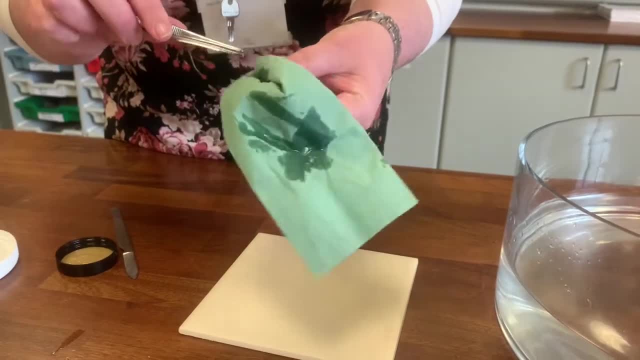 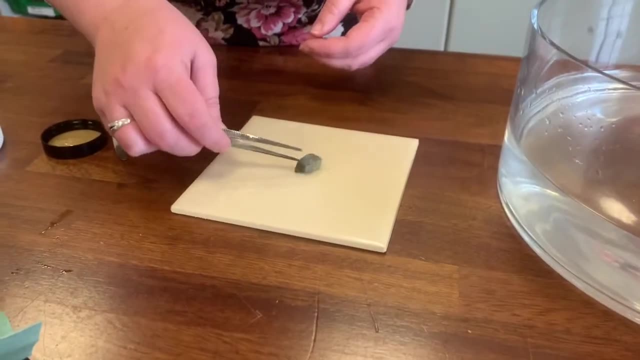 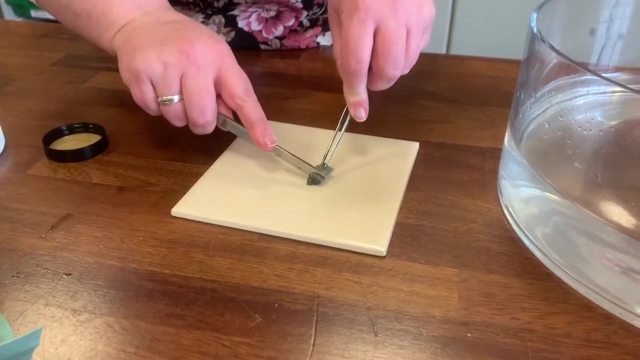 None of those are true, for well, actually they are shiny when they're cut, but then they react with oxygen. So let's see with the potassium. Again, it's just very dull at the start. So I'm going to watch, watch, how easy it is to cut and then watch how quickly this goes dull compared to the other two. 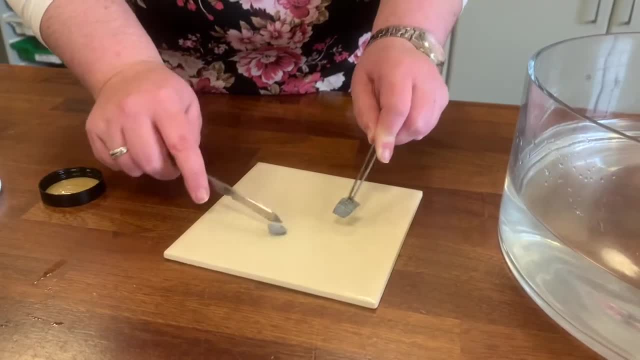 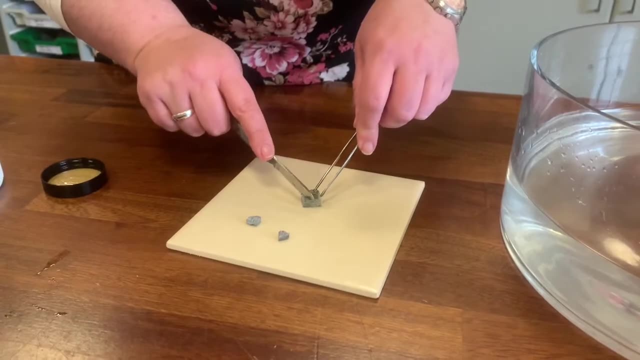 Probably dull already, is it? So that's just so. I'll do three bits of this one as well. So another part of our risk assessment is that there's a limit to the size of piece, So I'm only using very small pieces of metal. 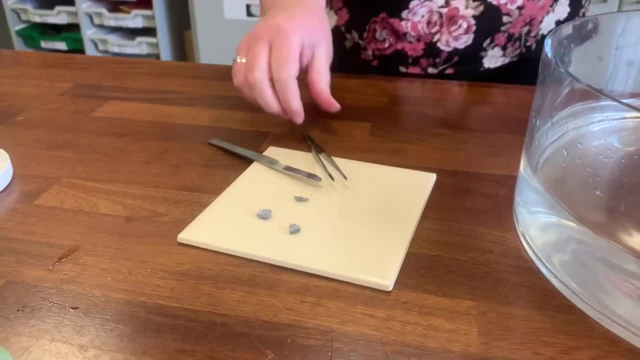 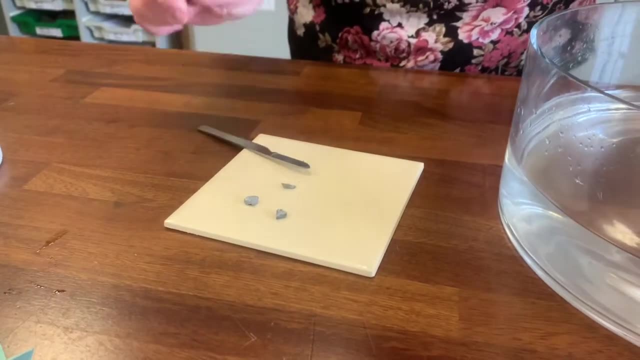 So, if I just go over the points of our risk assessment, we're wiping off the oil, We're making sure that the bottles are all clean, They're closed and out of the way before I put the metal into the water. We're using a very small piece. 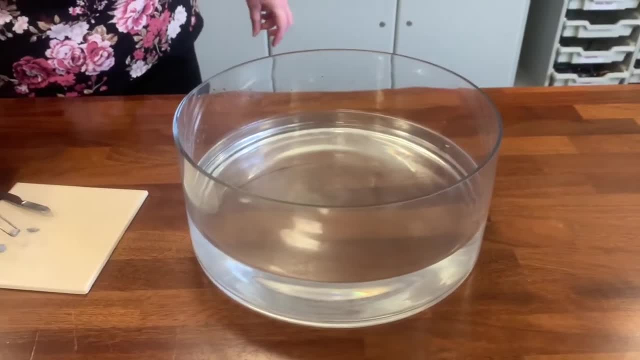 And when I put it in the water I'm standing back. So watch, with the lithium It's a bit different in the other two because we're getting further down the route, So it's more reactive. So watch what happens when we put lithium in. 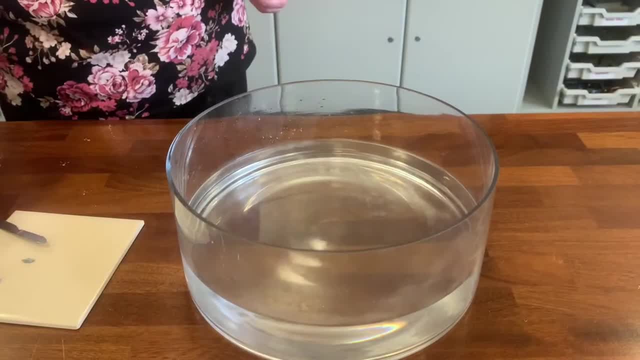 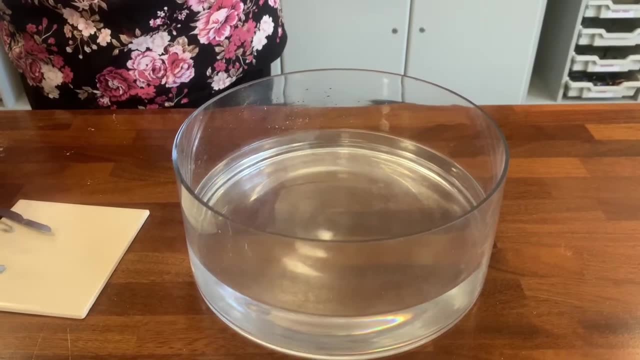 Pretty cool, eh. So our observations for lithium: It caught fire, didn't it Turn to the lilac flame? So when we do our flame tests we know the flame test for potassium is a lilac flame. It fizzles. 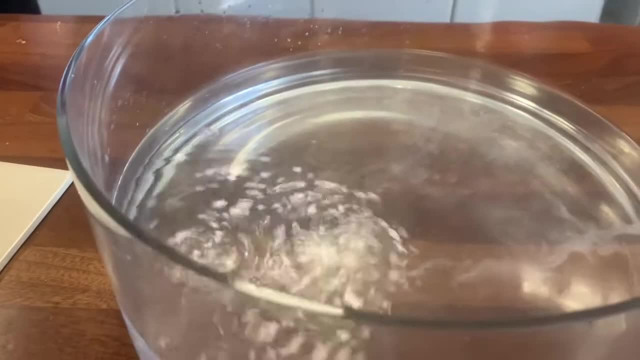 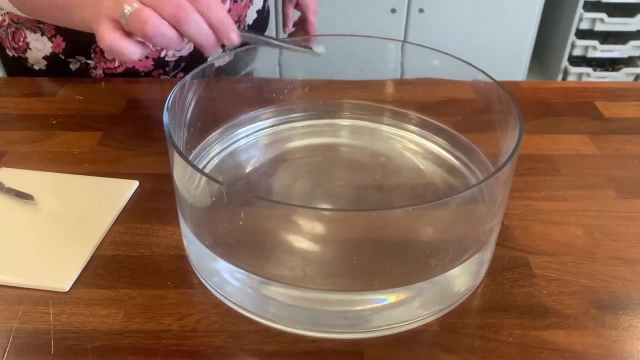 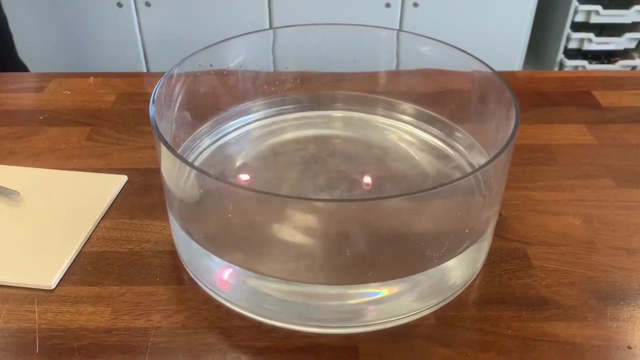 It fizzes. You can hear the fizzing, It can spark, It floats on the surface And we can definitely see the liquid going cloudy this time. And our last piece of sodium potassium. Oh, hopefully they're gone. And then our equation for potassium. 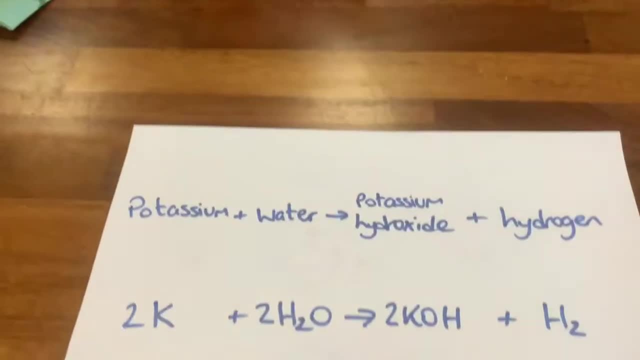 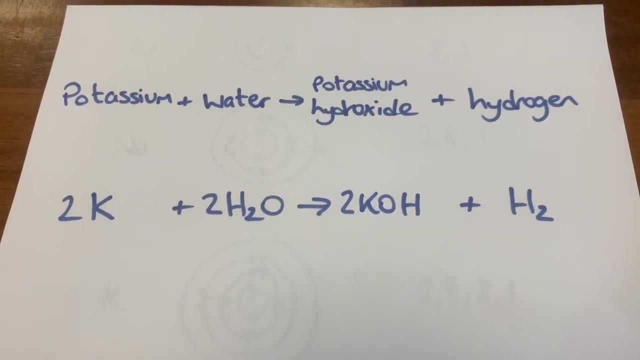 When it's potassium plus water, it goes to potassium hydroxide plus hydrogen. So again, those equations are very similar, Similar equations there as well, And the reason that they're called alkali metals is that they produce this hydroxide. 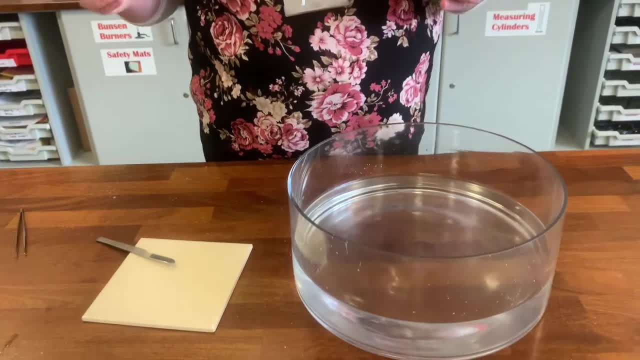 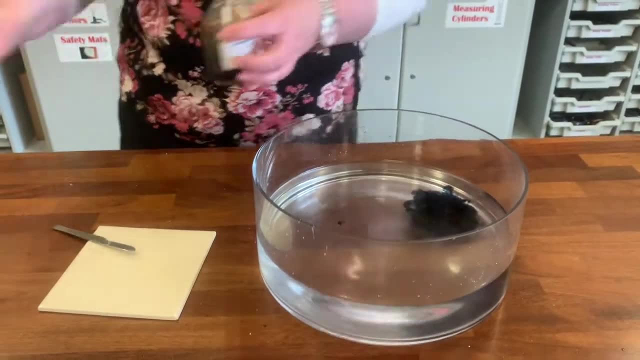 So the lithium hydroxide, the sodium hydroxide and the potassium hydroxide. So if you remember back to our pH scale, what acids and alkalis are, School bell going in the background. So when we add the universal indicator to it, it's going to tell us what acids and alkalis are. 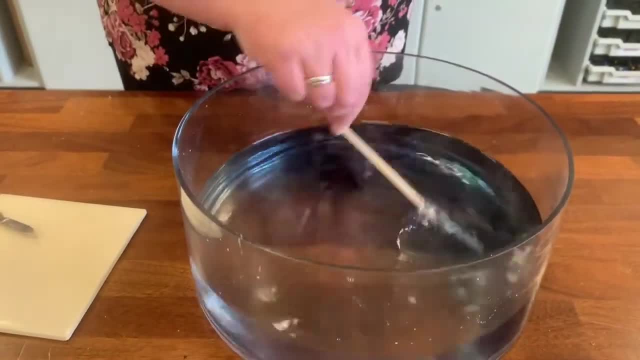 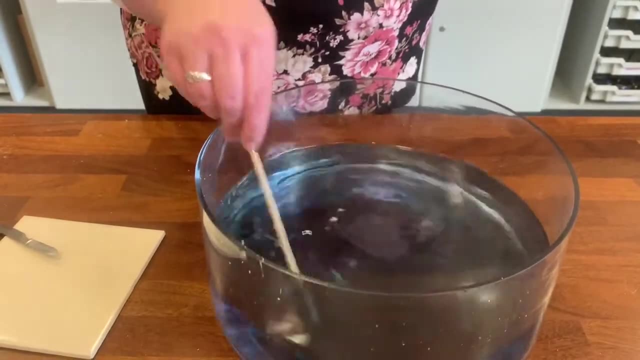 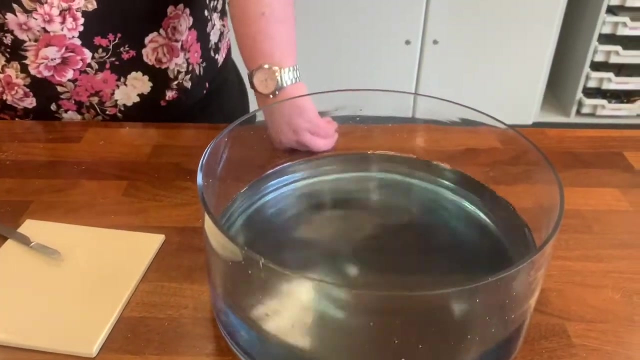 We can see that the water, which started off as neutral, has turned to a dark blue colour. It has a mixture of sodium hydroxide, potassium hydroxide and lithium hydroxide, So it's produced in alkali when the metals have reacted with water. 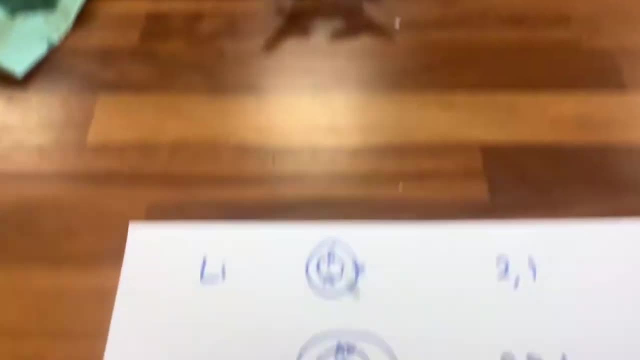 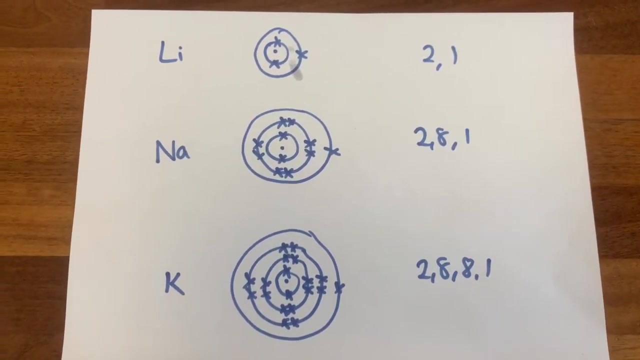 So the last bit I want to show you is just the electronic structure of the three metals. So they're all in group one, They all have one electron in it, or the shell. But as you go down the group they get more reactive. 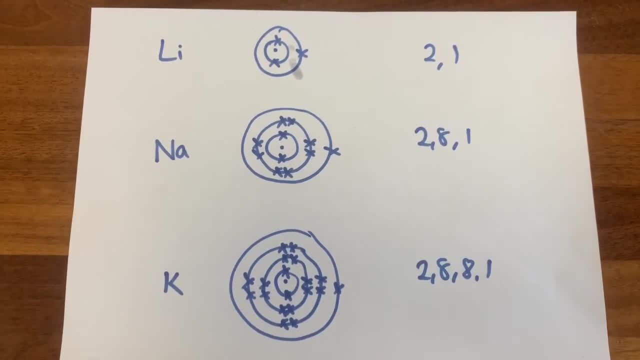 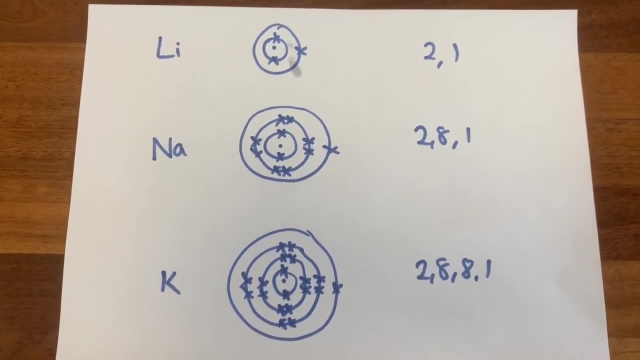 I want you to think back to that, Think back to what we were talking about when we did the electronic structure And just have a think and see whether you can describe why they get more reactive in terms of that outer electron. 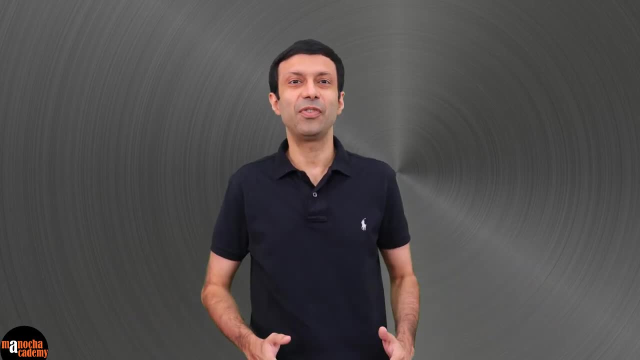 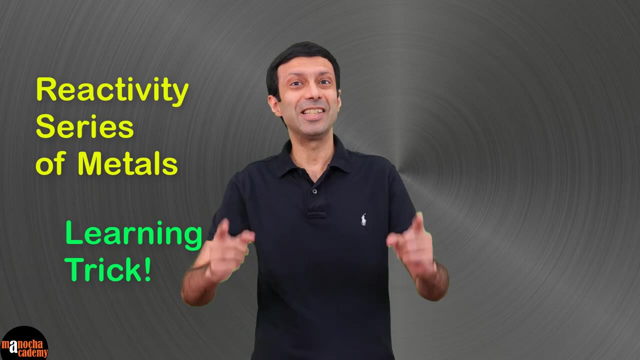 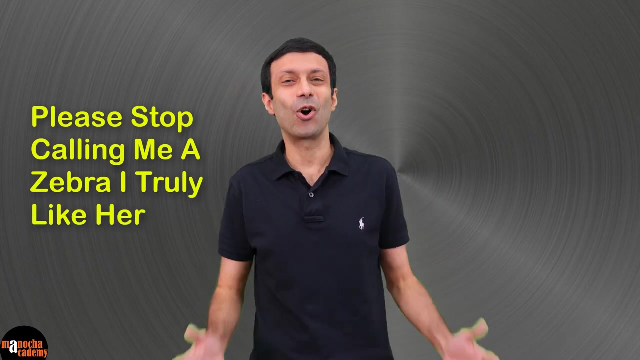 Hi friends, are you ready to learn reactivity series of metals in a way that you will never forget for the rest of your life? Here is the special mnemonic. Please stop calling me a zebra. I truly like her calling me super powerful giraffe. You must be thinking that's a song of. 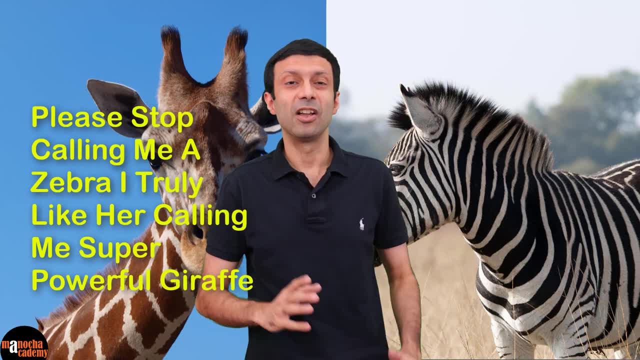 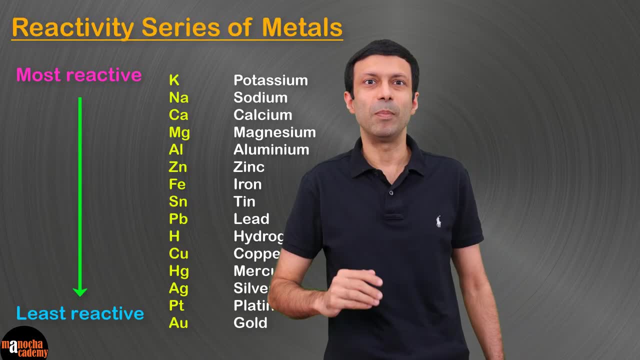 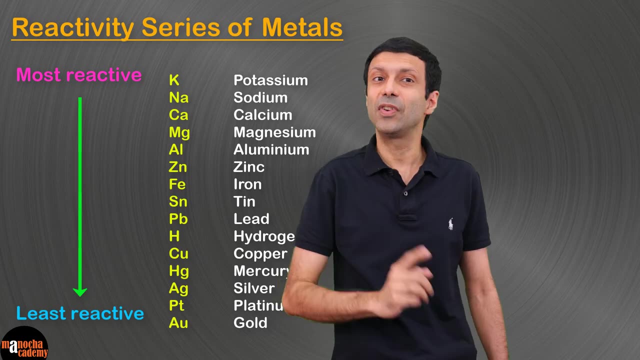 animals. Let's see how this mnemonic will help us remember the reactivity series of metals. Metals are arranged in a reactivity series, with metals of high reactivity at the top and metals of low reactivity at the bottom, So reactivity of metals decreases down the list And our mnemonic.